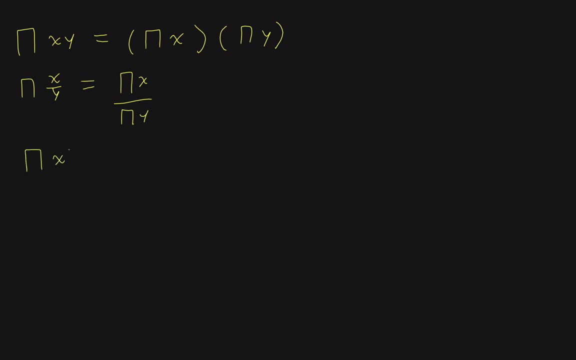 whatever that is. What if you have a power here? Well, let's take a look at an example of how this can apply. So you have 2 squared times x squared times y squared. Well, this is just the same as 2xy squared. 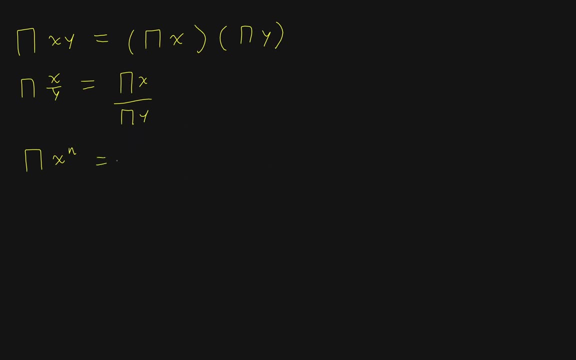 So what we can do With our product. that's going to be the same thing here. You can just basically take the power out. It's going to be the power of the products. So, product of whatever x is to the nth power. 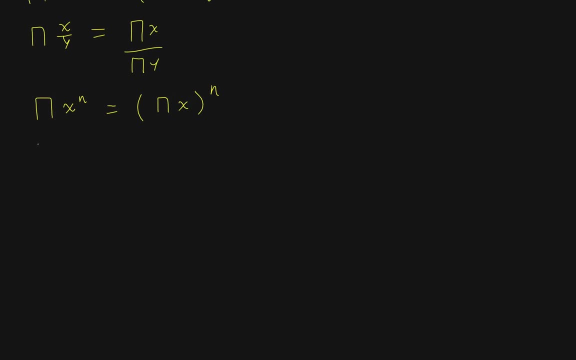 Now we're going to get to some of our standardized definitions. We have product, say, k equals 1 to n of k, Or the product of k equals 2 to n of k. Well, this is just going to be n factorial. You saw that above with the little example. 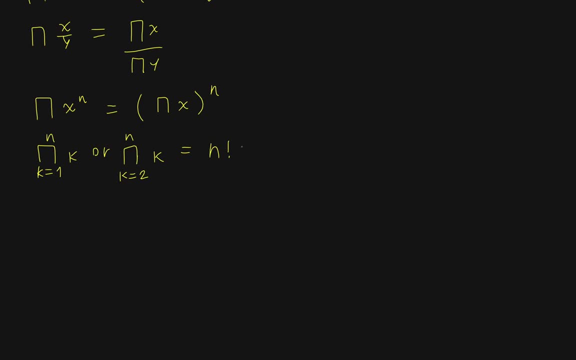 that we had here. So this is kind of the quote-unquote base case for product notation. Just like for summation notation you have n times n plus 1 over 2 for the base case. Here it's just n factorial for product notation. 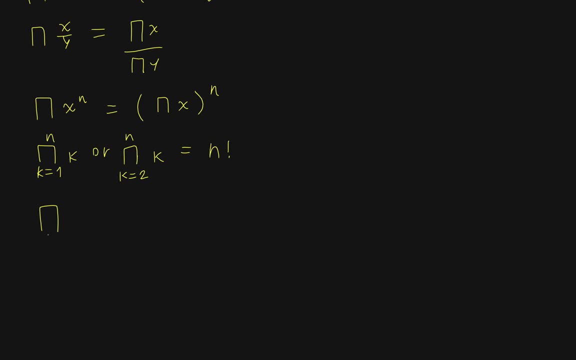 And so now, this is somewhat trivial, but something to keep in mind. If you have anything with a zero within the bounds, Like what, Like this: k equals 0 to n, or k equals m to some 0, where m is just going to be less. 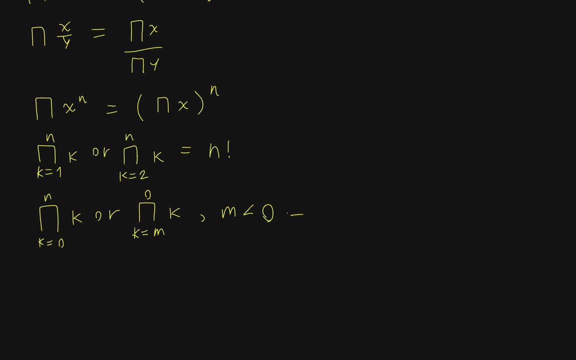 than 0. Then this is just going to be equal to 0, because 0 times anything is 0. Again, somewhat trivial but important to keep in mind. Now, how about a product isn't so nice? Let's say we have a nice starting index at 1 or 2 or anything like that. If we have product, 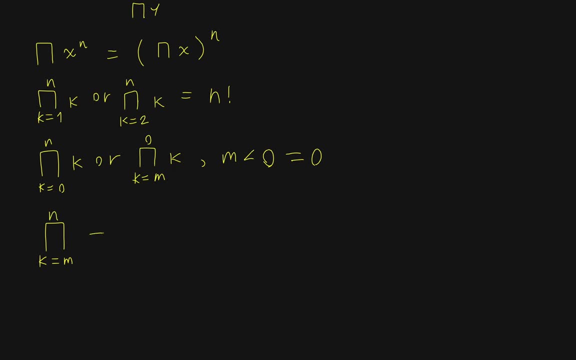 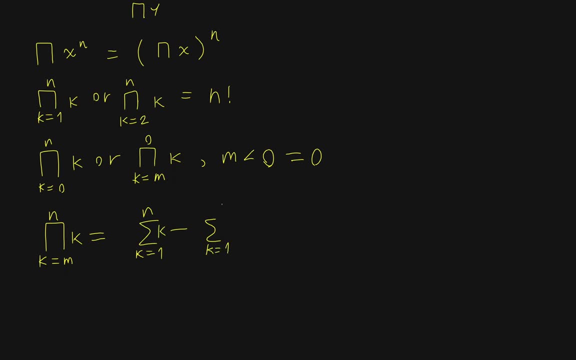 So that's the sum of k equals 1.. Put that k there- I almost forgot that- To m minus 1.. And it's a very, very similar structure or method for product notation. For product notation, you just start. so product of k equals 1 to n of k. 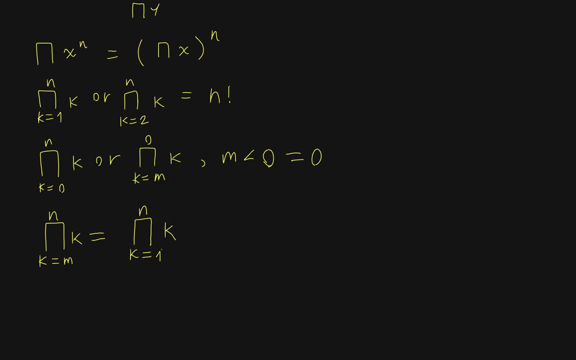 Now in the summation, basically you'd have addition And it's inverse is subtraction. Okay here for multiplication versus division. so we're going to divide by the product: k equals 1 to m minus 1 of k. so pretty much the same thing here. you just have the different kind of product. 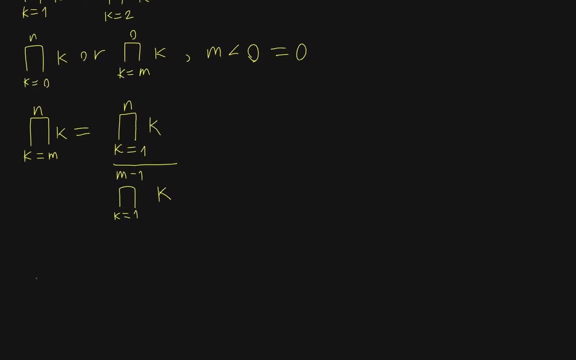 principles. the last one here is if you're dealing with a very tricky product that you can't really seem to simplify nicely, you can actually convert it to a sum. so if we have any product here, product effects whatever- then if we take the logarithm of the product- i'm just going to use natural log for 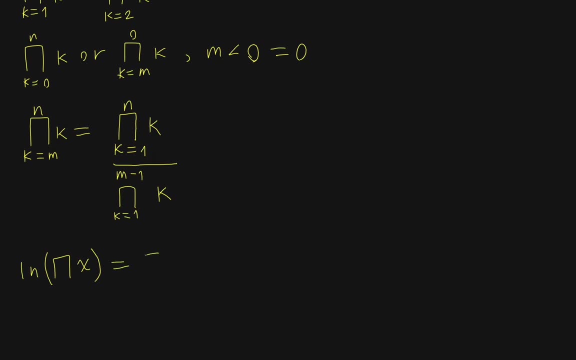 convenience here, then this is just going to be equal to the sum of the individual logarithms of the logarithms of the individual items, given the product law of logarithms. and then this also goes further, so that you can rewrite any product as, whatever your base is, here it was e to the sum. 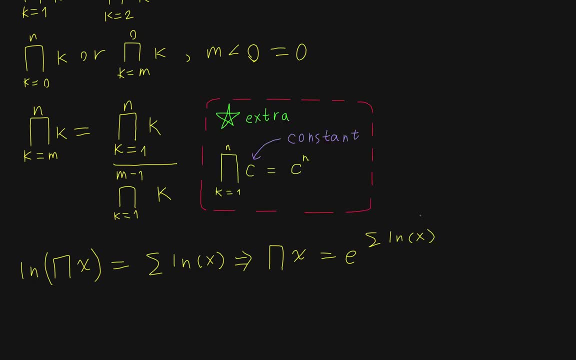 of logarithm of each of the items, one last one i missed, for constants. so these are the rules. now we're going to go over a couple of examples here. all right, so let's start a little bit simple. we're going to have product. it's going to be x. squared from x equals three to seven. well, 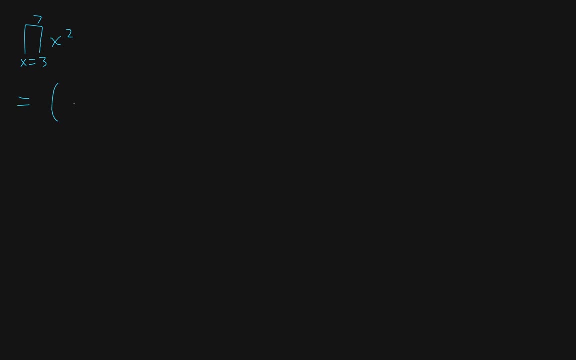 first of all, you notice, we can take the power out over here. so we're going to have product x equals three to seven x and this is all squared. now again, these do not start at uh. the bottom, uh bound does not start at one. so we can reset the index and have product x equals one to seven of x over. 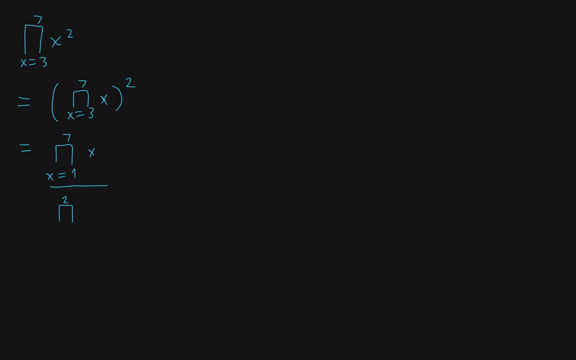 the product of uh. three minus one, that's just two. x equals one of x. this is again all squared Now. here we can rewrite this as factorial. so we're going to have 7 factorial over 2 factorial squared. Now we can basically expand these factorials. 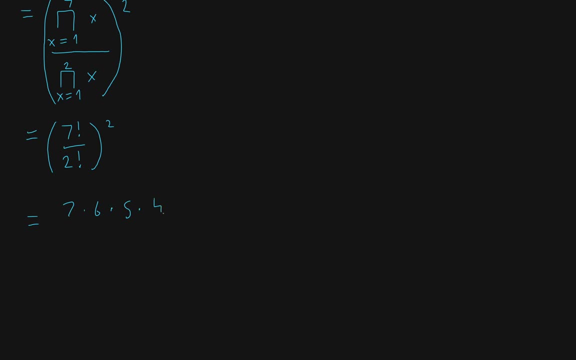 if we want, We have 7 times 6 times 5 times 4 times 3 times 2 factorial, all over 2 factorial, and this is once again squared. Now, over here, these guys are going to cancel out. so we are just going to have 7 times 6 times 5 times 4 times. 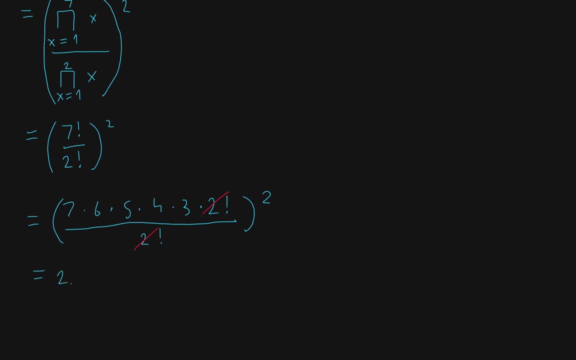 3 squared, that is going to be 2, 5, 20 squared, and then it's going to be a big product. here It's going to be 6,, 5,, sorry, 6, 3, 5,, 0,, 400 in the millions here. 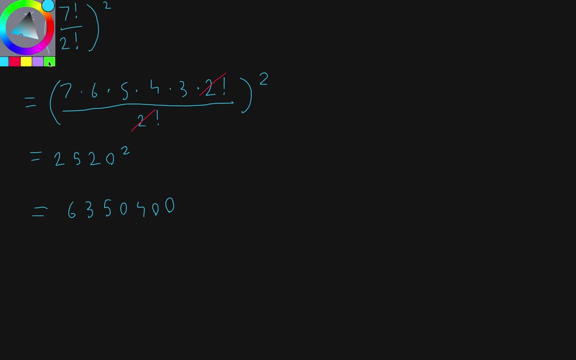 So that is the final answer over here. Just box it in like that. Okay, now let's take a look at a bit of a more complicated example. We're going to have here a polynomial involved. It's going to be: product from x equals 2 to 6 of x squared minus 3x minus 10.. 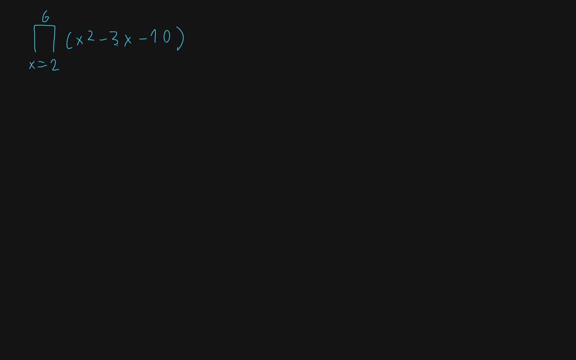 Now. so you have kind of like sums or any other arithmetic operations in here. You're going to want to try and find a way to separate these out. This is a quadratic and it's also nicely factorable, So we can separate these into two products of the individual factor. 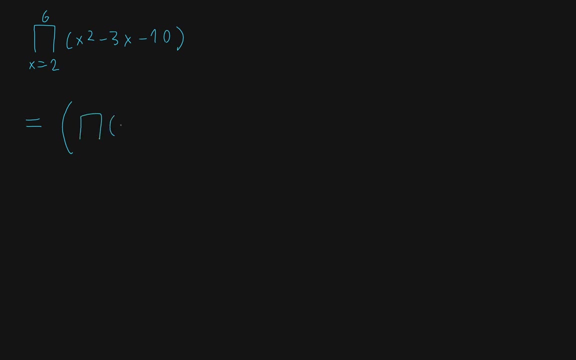 So this is going to be basically: you're going to have x minus 5 and then product x plus 2.. Same indices from x equals 2 to 6 and x equals 2 to 6.. Now from here, technically, if you have simple kind of, 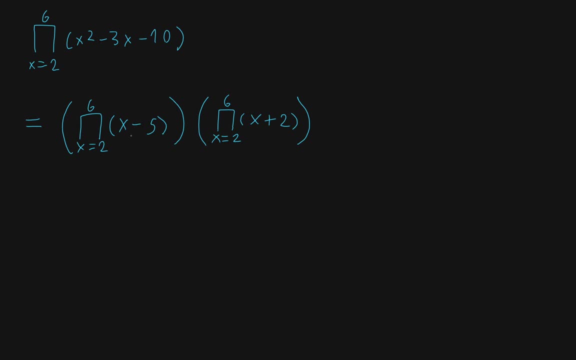 sums in between. like this you can. there's a sort of way to expand to a certain kind of unit polynomial, but that's quite complicated And what we're going to do here is just change it to summation. So I'm already going to put this to exponential. 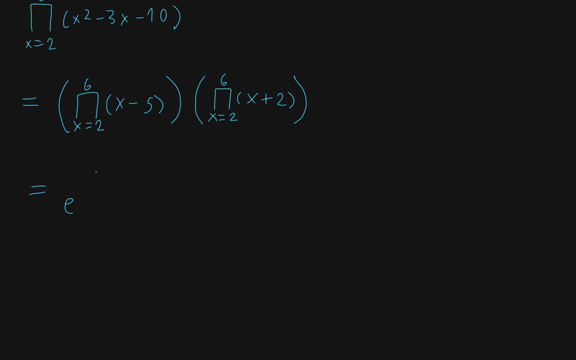 So here, use natural log again. You're going to have e to the sum x equals 2 to 6 of natural log x minus 5, and then plus this sum again, x equals 2 to 6 of the natural log of x plus 2.. 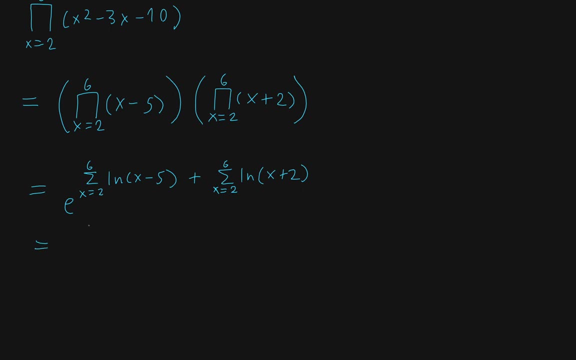 Now, with these guys, their indices are quite small. We're going to have to kind of calculate them manually. But here what you're going to have is e to the natural log of 0, and then plus here 2 plus 2, that's going to be 4 to 8, so 4 to 8 all multiplied. 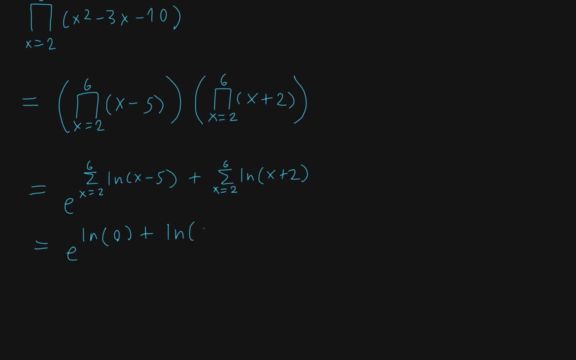 is going to be natural log of 6,, 7,, 20.. Now over here we have to consider this log of 0 as a limit. So if we're going to have, we're going to have ln of 0 plus right. 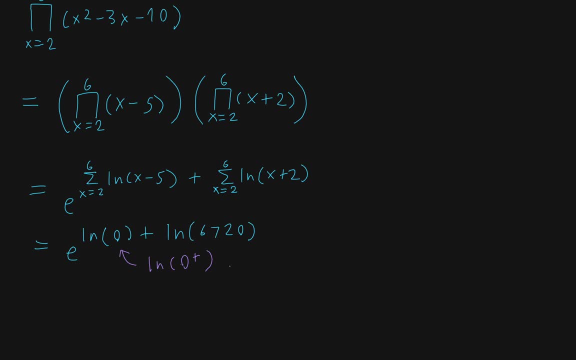 because we're not considering a complex definition here. so this is going to be approaching negative infinity infinity, which also means that this right over here is going to be insignificant. Now we're going to have basically e to the negative infinity, which is just 1 over e to 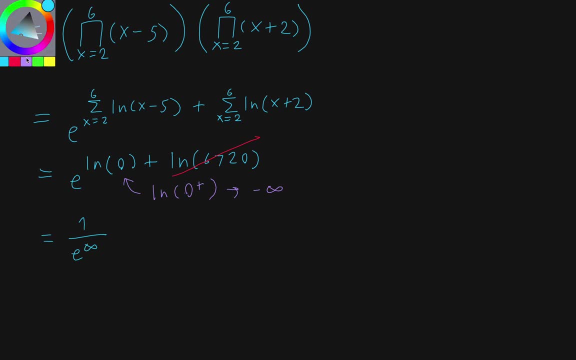 the infinity. Now, this bottom denominator over here is going to go towards infinity. so basically you're going to have 1 over infinity which is going to approach 0, and that is our answer. it is going to be 0.. So at one point one of the partial products was 0 and that basically made everything else. 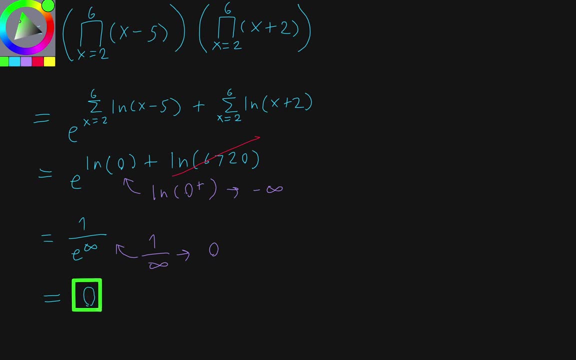 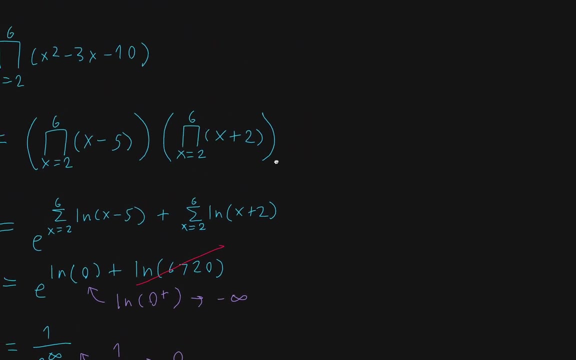 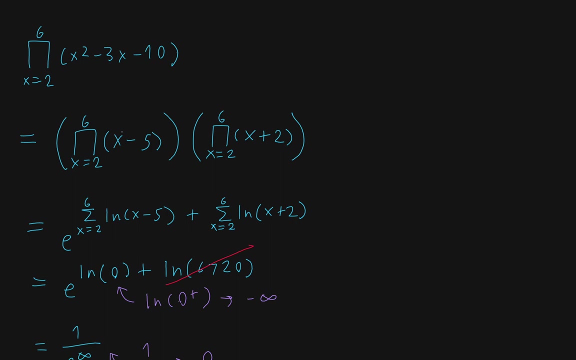 0.. I'm just going to box this in Now. let's look up over here A way that we could have basically shortcutted this is that you have a polynomial here, You have the factors. You can see here that we're going to hit one of the x-intercepts, which means that at least